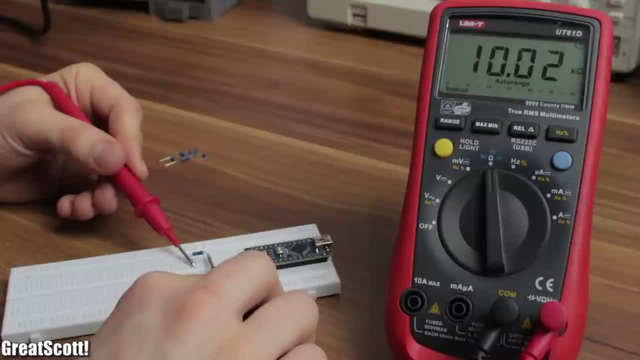 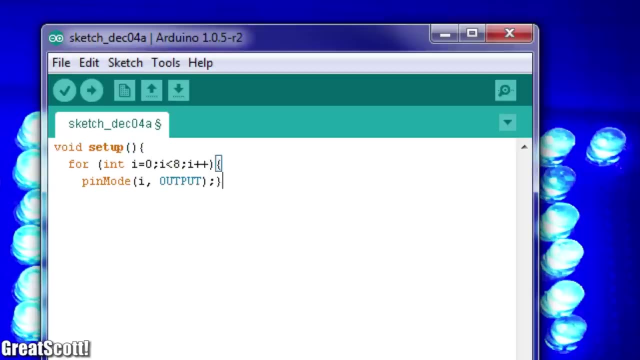 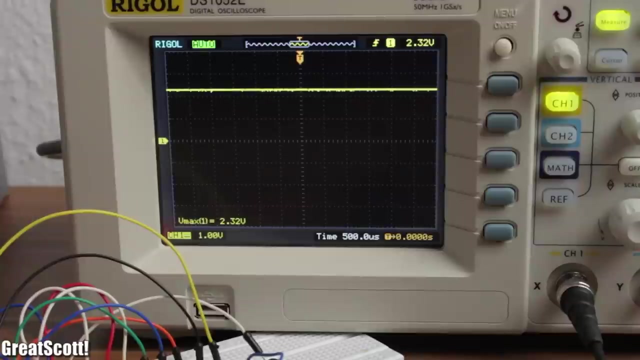 explaining. I will now build this DAC here with 10k resistors and 20k resistors. Now let's experiment. I put pin 7 high and all the other pins low. Here I'm using the port D command to set the voltage output level. It is just faster this way And we get around. 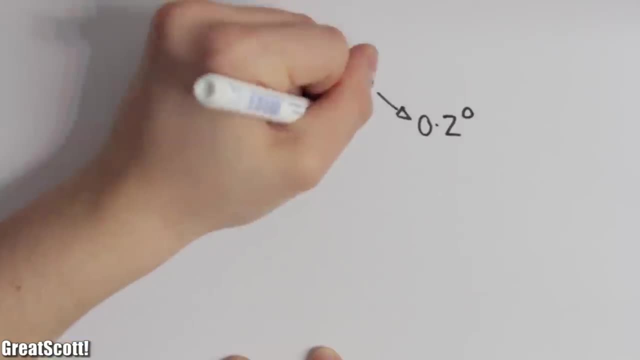 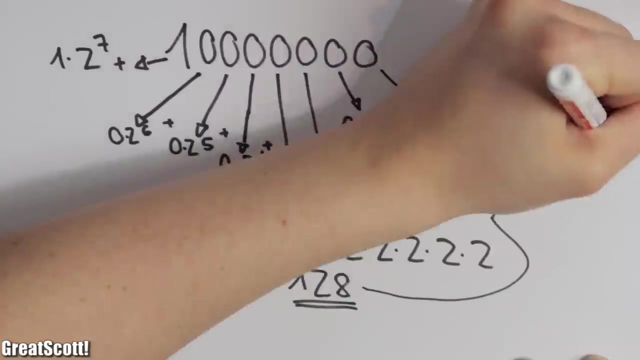 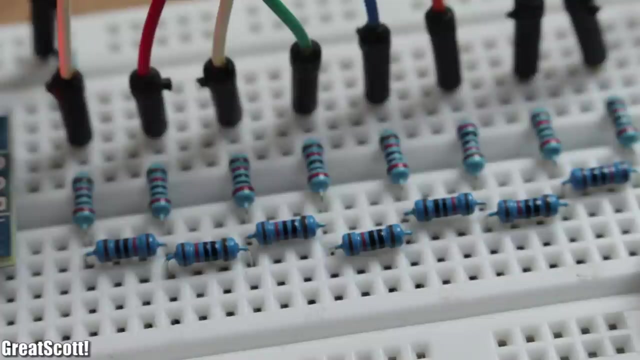 2.3 volts on the output. If we convert this binary number into decimal, we can see it is the number 128, which is exactly the half of 256.. And 2.3 volts is around the half of the max voltage, 4.8 volts. It is not precise because these resistors still have a 1% tolerance. 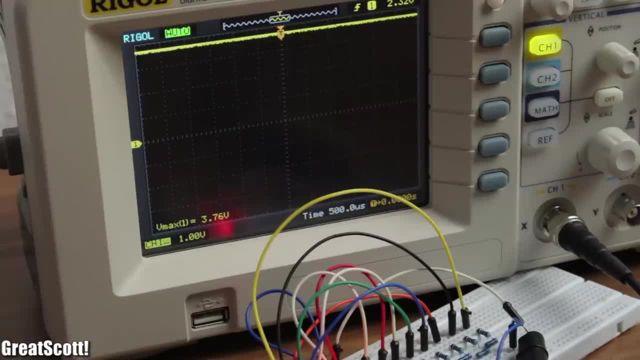 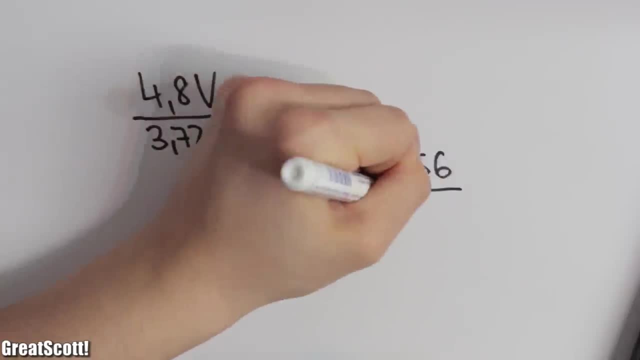 Now let's try the number 200. And we get around 3.72 volts at the output. 4.8 volts divided by 3.72 volts is around the same as 256 divided by 200. I think now you get how this works With this knowledge. 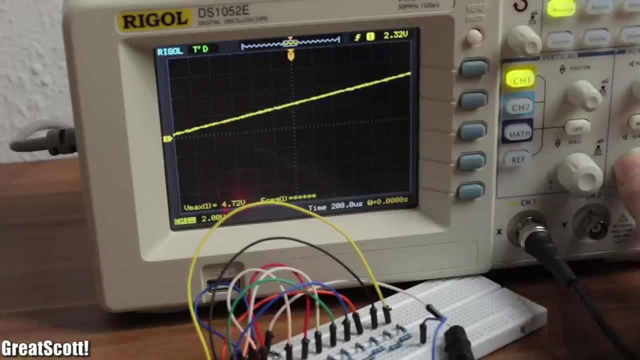 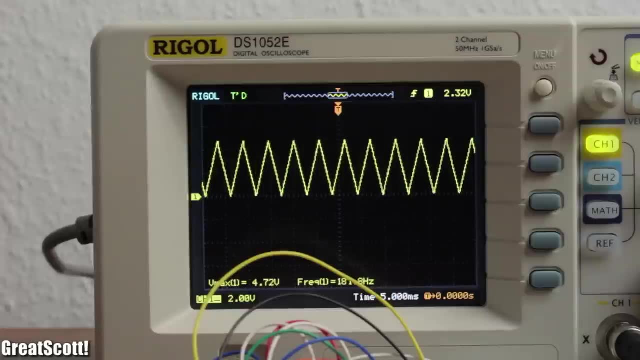 we can easily make a ramp function by slowly increasing the port D value up to 255, and then going back to 0. Or a triangle function by increasing port D to 255 and then decreasing it back to 0. If we zoom in a bit, we can still see that there are steps between voltage levels and 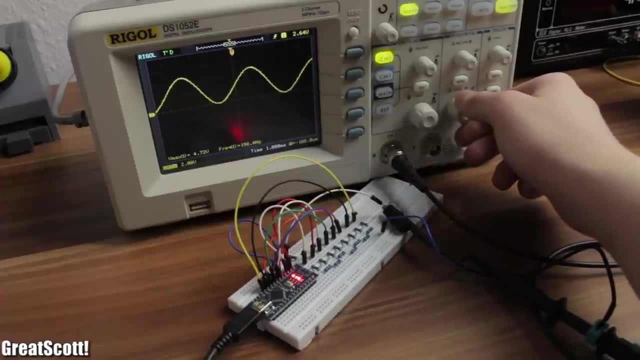 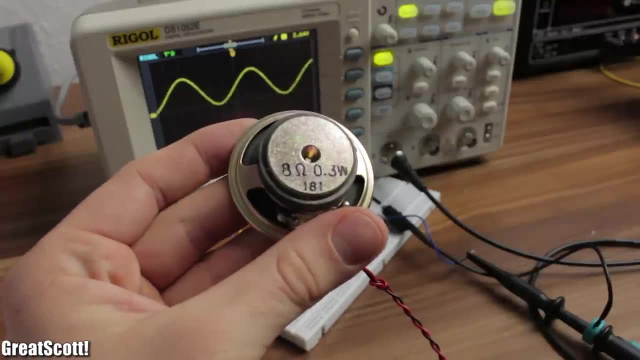 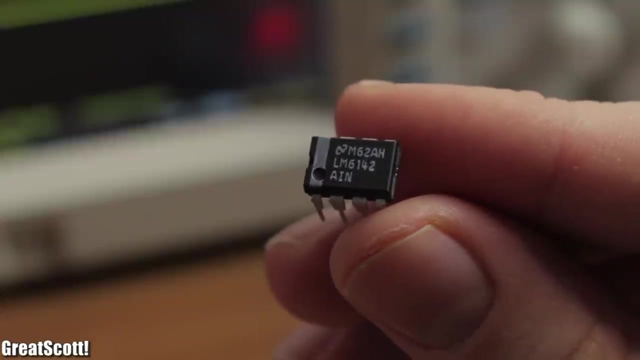 no smooth flow, But let's have some fun with a sine wave. now, If we want to hear this signal, we could connect a speaker right. Well, you cannot connect this directly to the resistor ladder because the voltage will collapse or change its form completely, So we have to use an op-amp as 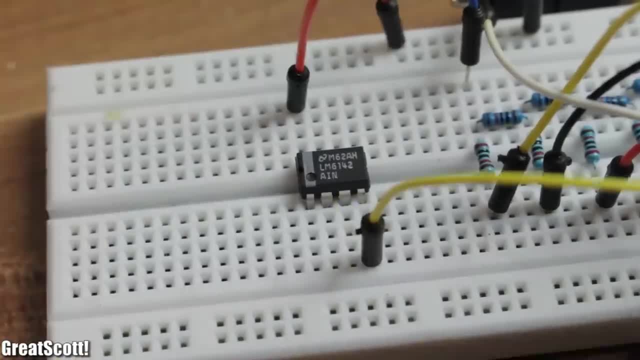 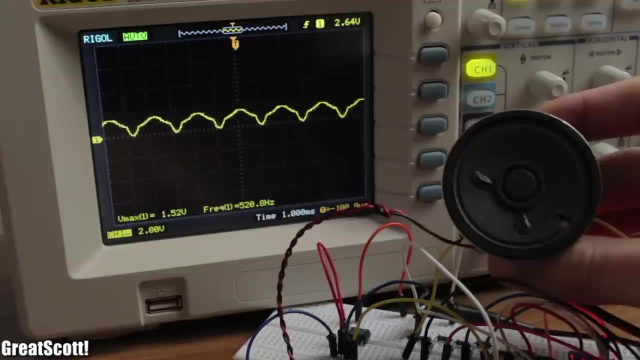 a voltage follower. It does not amplify the signal, it just keeps the output voltage stable when we connect a load- Not a huge load, though, And now let's hear a 500 Hz sine wave, Or a 1 kHz sine wave, Or let's just go crazy. 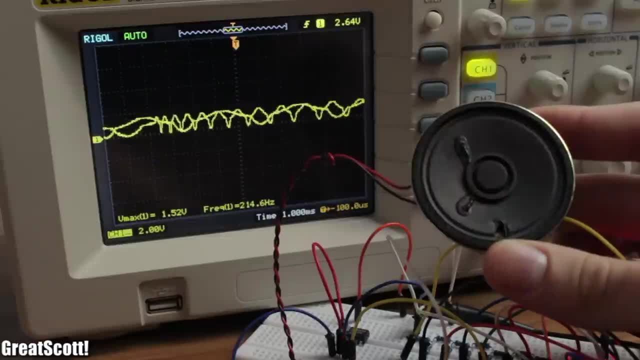 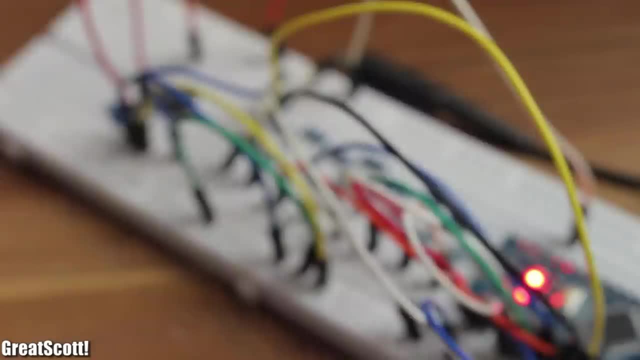 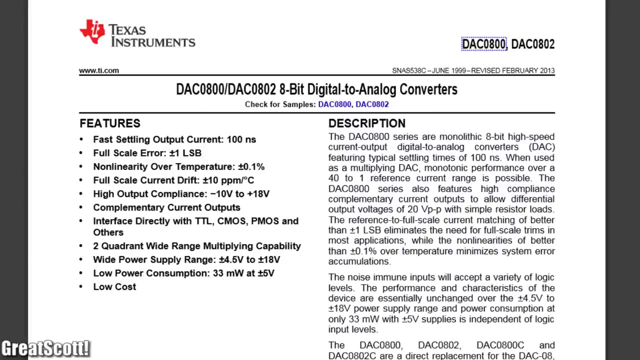 and hear a fast changing sine wave between 200 Hz and 3 kHz. I don't know why, but it kind of sounds like an Atari 2600 sound effect. If you want a more precise and small DAC which works the same way, then you can look for ICs which do that, like this DAC 0800.. 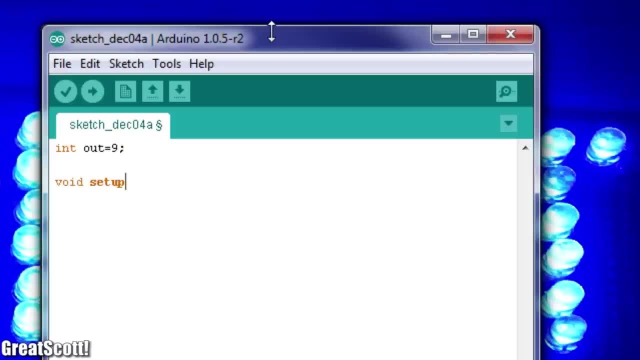 But some of you might already thought: why all this crap? The Arduino has an analog write function. Isn't that the same? Well, kind of It is also 8 bits. so let's try it with a value of 200 again, And we see. 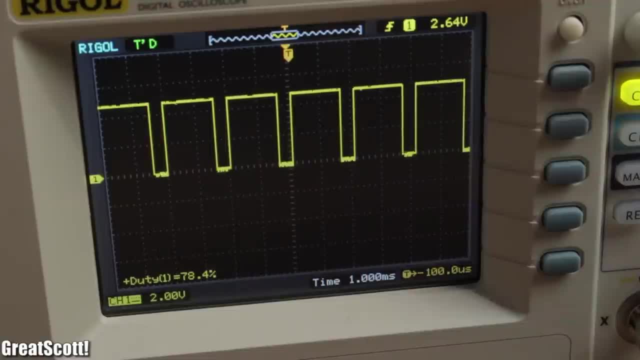 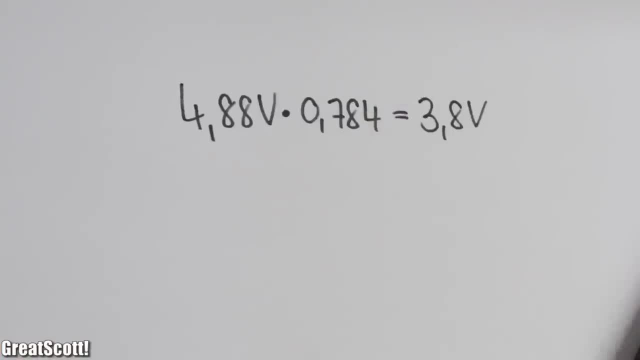 a PWM signal between 4.88V and 0V, with a duty cycle of 78.4%, which is an average of 3.8V, which makes sense when we enter 200.. But here is the magic ingredient which makes: 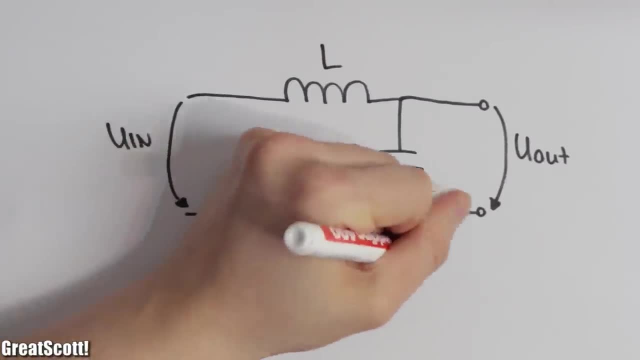 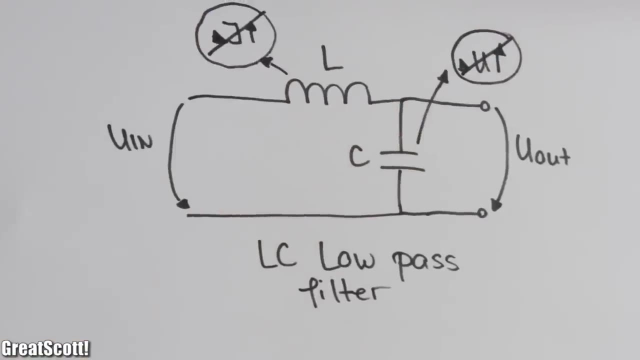 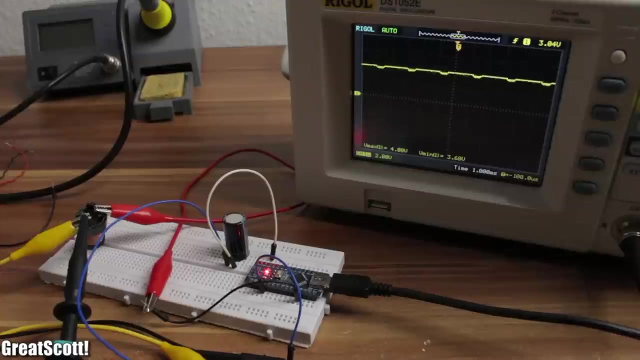 this into a DAC. It is called a LC low pass filter. The coil resists sudden changes in current and the capacitor resists sudden changes in voltage. So together they make this bumpy write kind of smooth, And we can also increase the capacitance a bit to make this voltage. 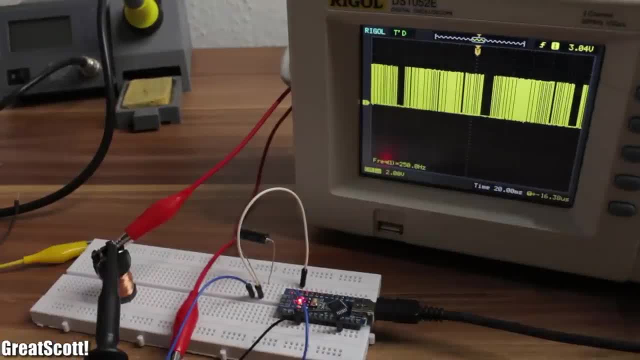 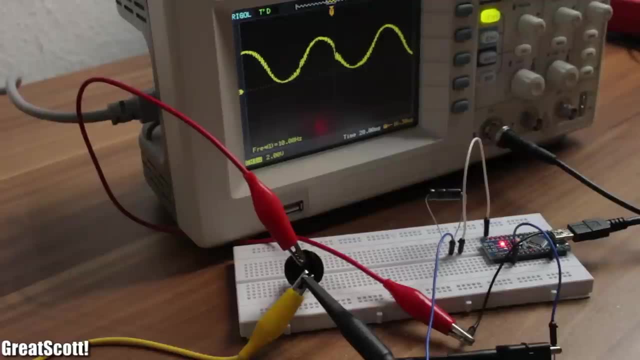 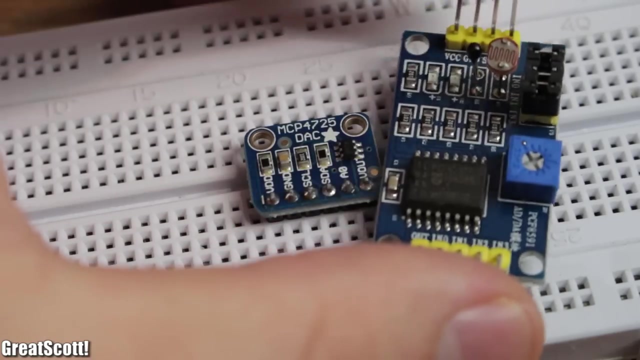 more stable. Now let's try the sine wave. Here is it. without the LC filter You can't even tell what it is supposed to be. And here is the voltage with the filter. Pretty awesome, I guess, But not so easy to use. Much easier to use would be these I2C devices. They only need two pins. 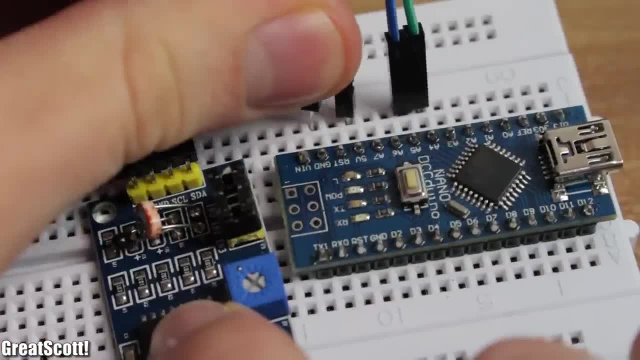 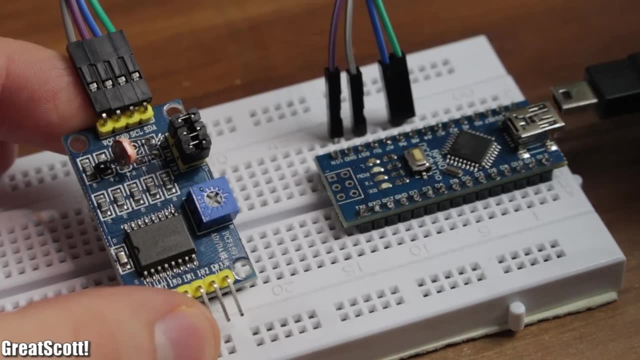 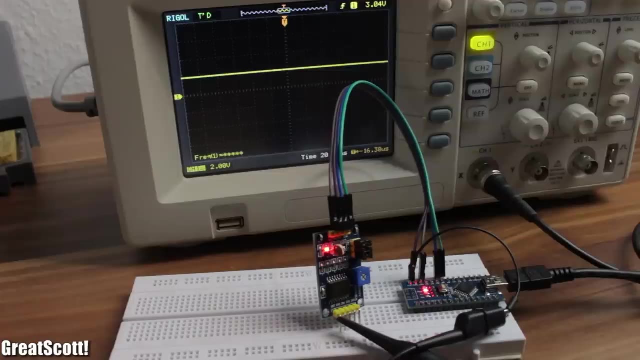 of the Arduino serial data and serial clock which connects to pin A4 and A5. Then all you have to do is send your analog value over to them and they do all the work by themselves. I have this PCF8591 8-bit DAC from China and it works great. And if you want an even better, DAC, you can take a look at Adafruit's MCP-4.. So let's try it out, And here is the result. It works great, And if you want an even better DAC, you can take a look at Adafruit's MCP-4.. So let's try it out, And here is the result. It works great. And if you want an even better DAC, you can take a look at Adafruit's MCP-4.. So let's try it out, And here is the result: It works great. And if you want an even better, 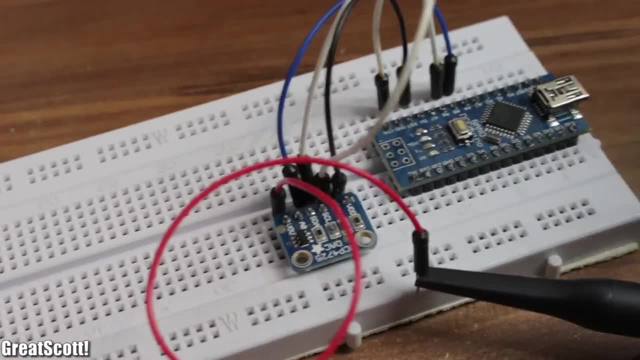 DAC, you can take a look at Adafruit's MCP-4.. And here is the result. It works great. And if you want an even better DAC, you can take a look at Adafruit's MCP-4.. I guess now you know how a DAC works. They are used to produce analog audio and 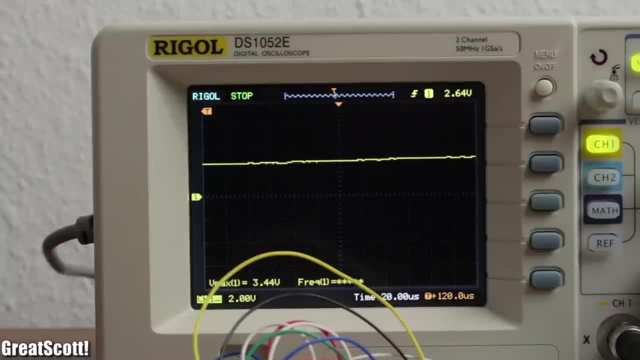 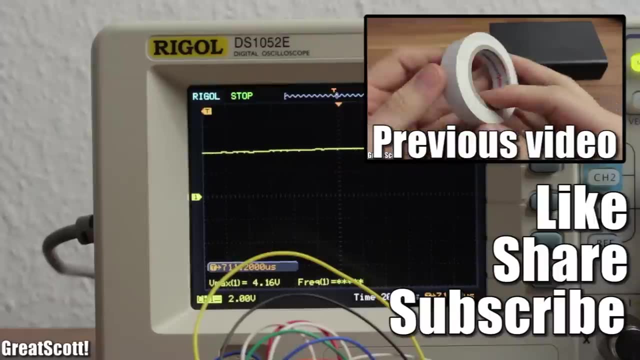 video and are also useful to build a frequency generator or to test audio filters. Let's see what I will build with them in the future. As always, dont forget to like, share and subscribe. Stay creative. stay creative and I will see you next time.